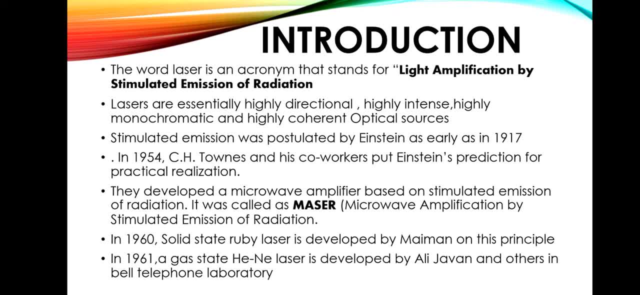 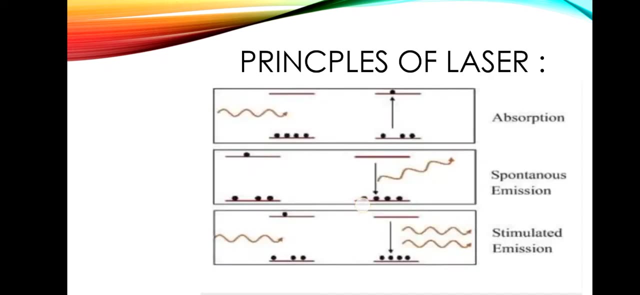 Maimon built the first laser laser system in the world laser device and in 1961 Gastate helium-neon laser is developed by Ali Chavan and others in Bell telephone laboratory. some lasers generate visible light, but others generate ultraviolet or infra-array rays which are invisible. 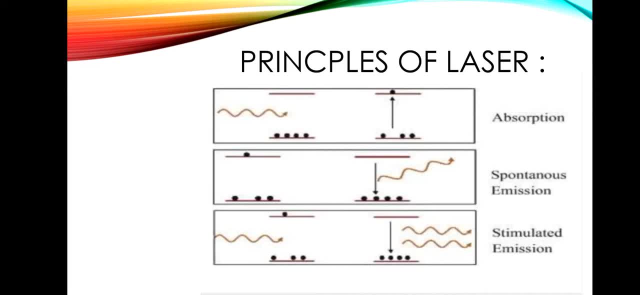 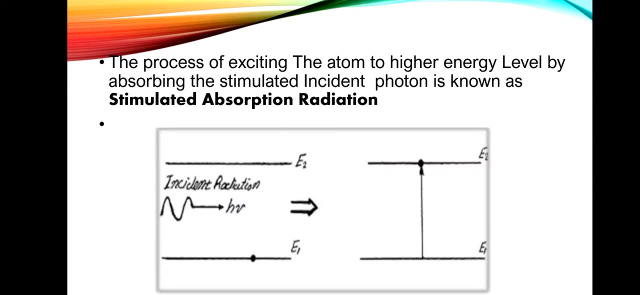 principles of laser. there are three principles of laser. they are: absorption, Absorption, spontaneous emission, stimulated emission. We will see one by one. First, absorption is also called as stimulated absorption of radiation. An autumn in lower level absorbs a photon of frequency and moves to an upper level. Here it is an autumn. This autumn, from lower level, moves to the upper level. 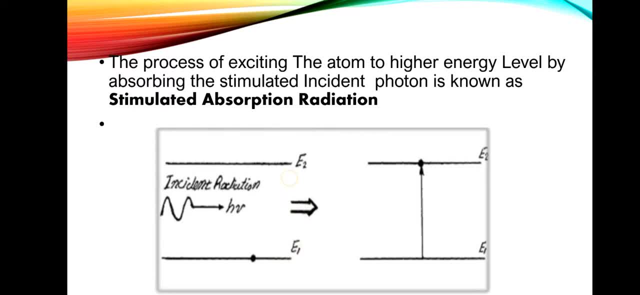 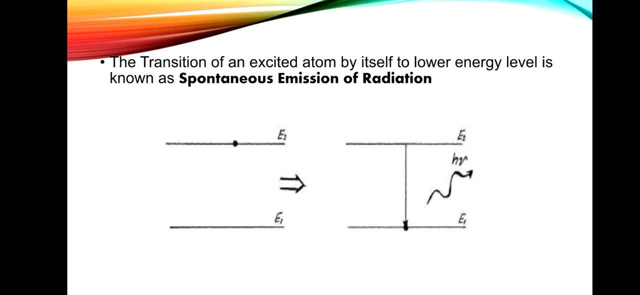 This autumn in lower level moves to upper level, It is called as stimulated. Stimulated absorption of radiation, Next spontaneous emission. The transition of excited autumn by itself to lower energy level is known as spontaneous emission of radiation. Autumn in an upper level can decay spontaneously to lower level. 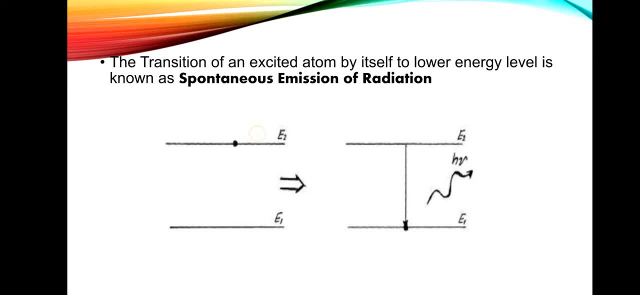 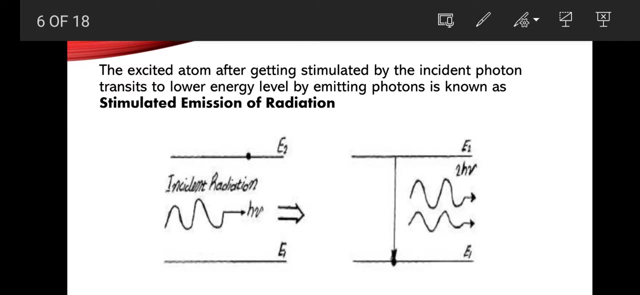 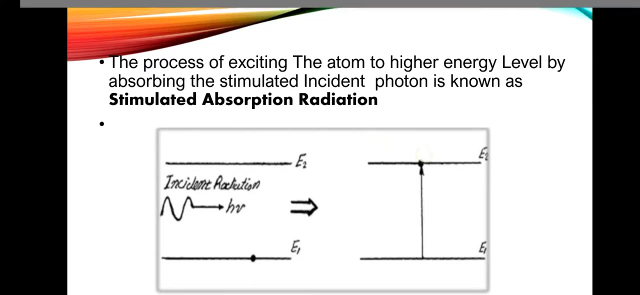 The atom firstly positioned in upper level spontaneously decayed to lower level. It was spontaneously decayed to lower level Spontaneously. the atom in upper level spontaneously decayed to lower level. Spontaneously decayed to lower level is called spontaneous emission of radiation. 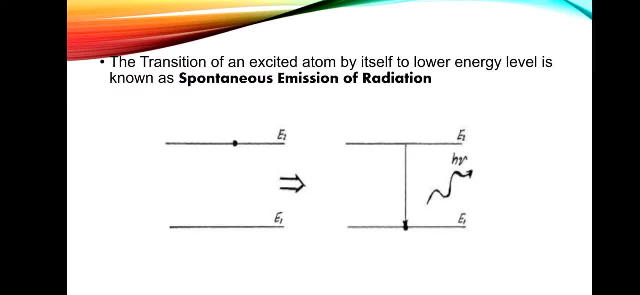 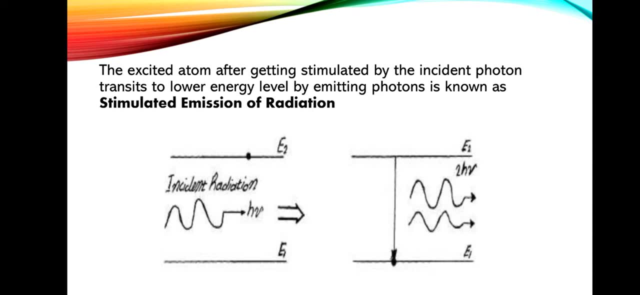 Next spontaneous, Next one: stimulated emission of radiation. Stimulated emission of radiation: The atom, after getting stimulated by instant photon, tenses to lower energy level by emitting photons. is known as stimulated emission of radiation. Here you see, And instant photon causes an upper level autumn. 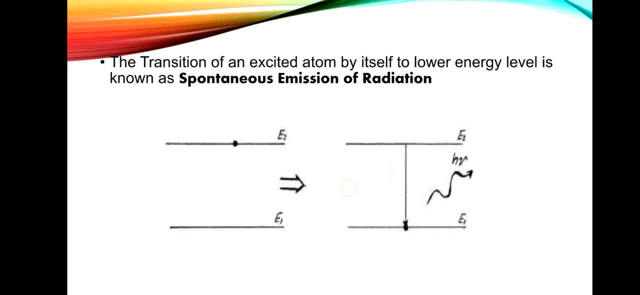 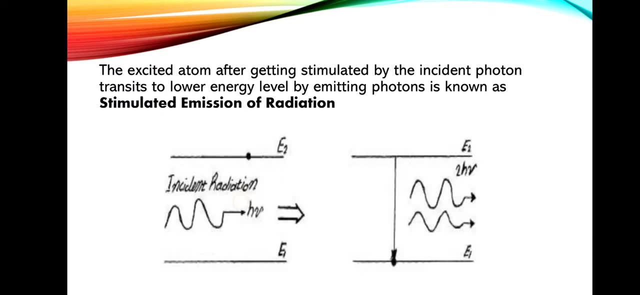 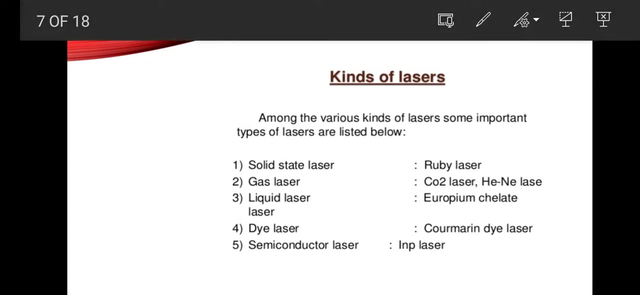 This incident. photon causes an upper level, the autumn, in the high level. Next one stimulated emission of radiation: current citizens in lower level. an upper level, the autumn, which is in upper level. it causes to decay. to decay and emitting a stimulated photon. okay, whose proper is, and emitting a stimulated. 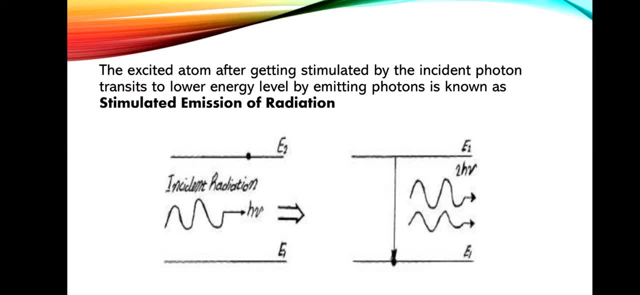 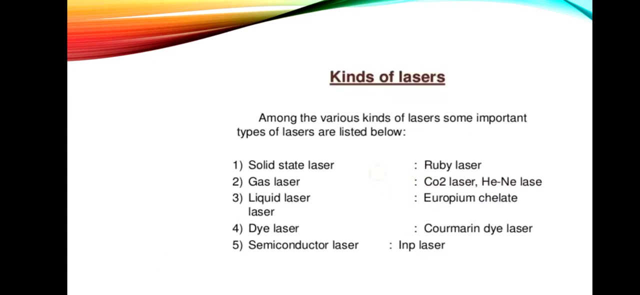 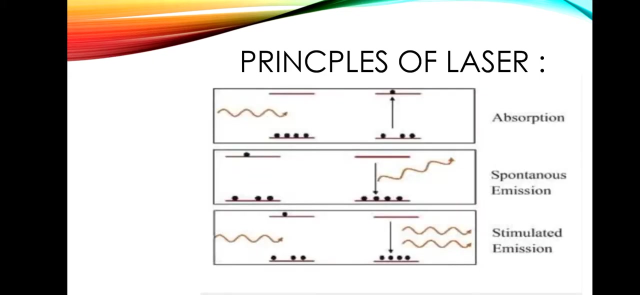 proton, whose properties are identical to those of instant photon. the term here, the term stimulated here, the term stimulated in underlines the fact that this kind of radiation only occurs if an instant photon is present. okay, next, these are the three types of radiation. these are three types of laser. these are: 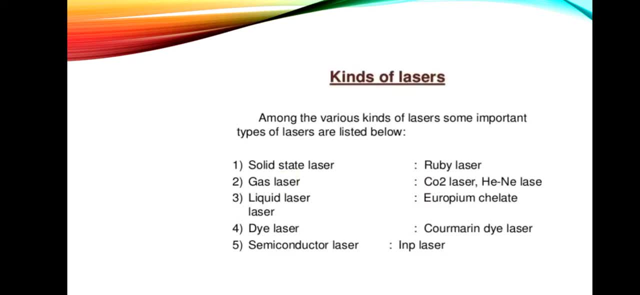 three principles of laser and next, kinds of lasers. okay, there are so many kinds of lasers here. some of the important lasers are listed here, like solid-state laser, gas laser, liquid laser, dye laser and semiconductor laser. in ruby laser is an example of solid-state and co2 laser, helium neon. 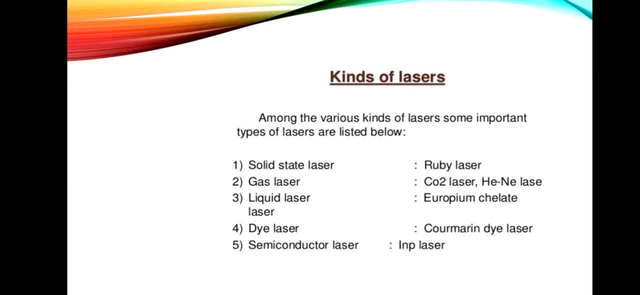 laser is an example of gas. europium chelate is an example of liquid laser. cormorant dye laser is an example of dye laser. here the word cormorant is new to us. it is a colorless crystalline solid with sweet order resembling the scent of 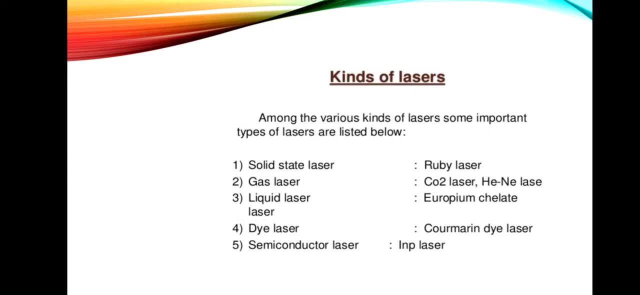 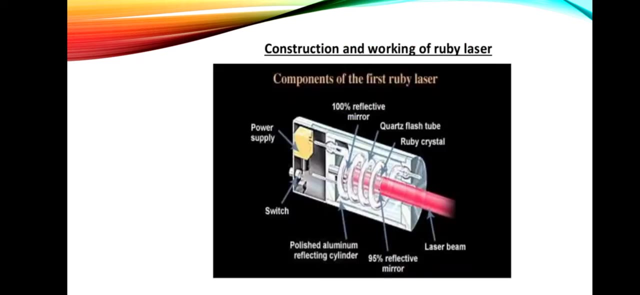 vanilla and a somewhat bitter taste. it is found in many plants too, and LNP is a semiconductor laser. LNP is nothing but lithium neodymium tetraphosphate laser. that is the type of semiconductor laser. next, here we'll see an example of solid state laser. there is ruby laser, the lässt. 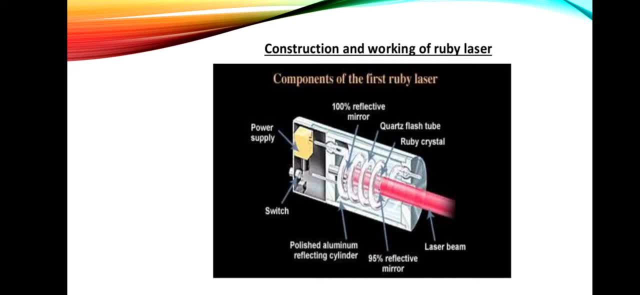 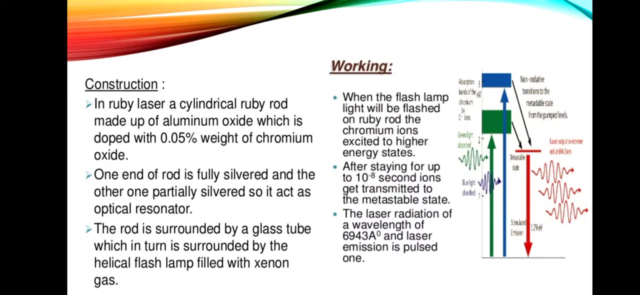 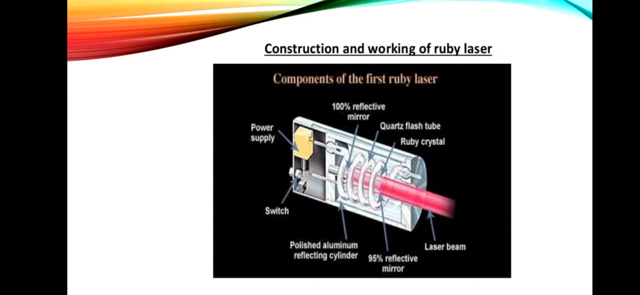 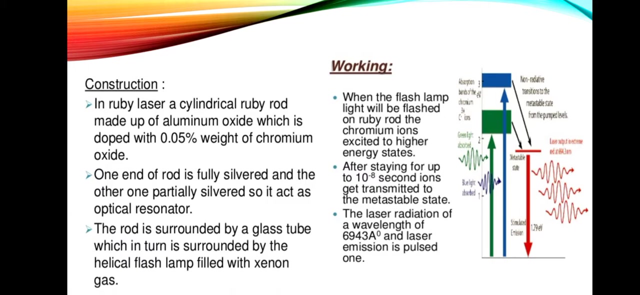 Here the construction of a ruby laser. A ruby laser is a solid state laser that uses a synthetic ruby crystal as its gain medium. Let us see its construction and working. Coming to the equipment, We will see the construction and working part. Let us see the construction of a ruby laser In. a ruby laser is a cylindrical ruby rod made up of aluminium oxide which is doped with 0.05% weight of chromium oxide. 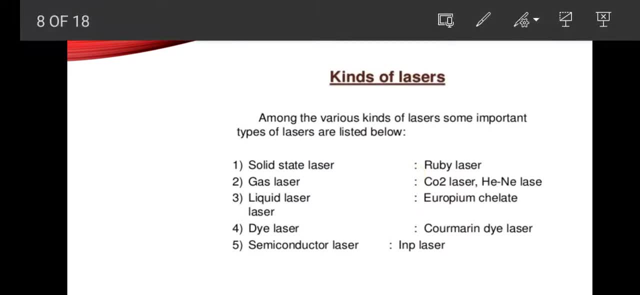 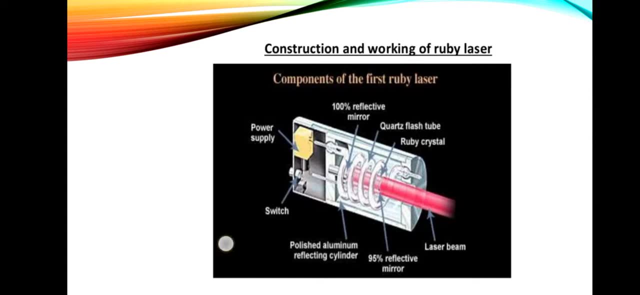 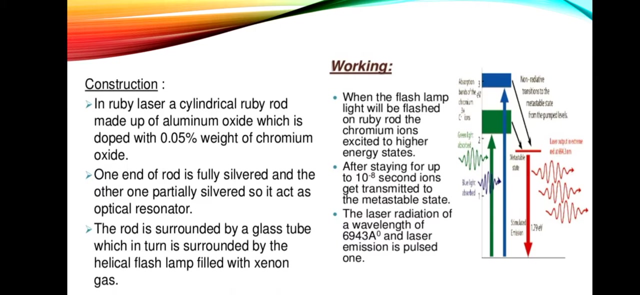 Alright is fully silvered and other end is partially silvered with aluminum. for optical. this optical resonator is used to build up the light energy in the beam. they are essential for the operation of lasers, and the rod is surrounded by a glass tube which in turn is surrounded by the helical. 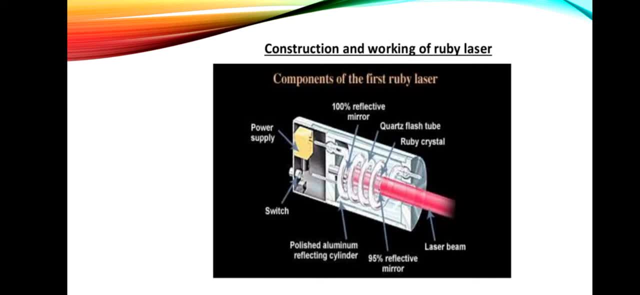 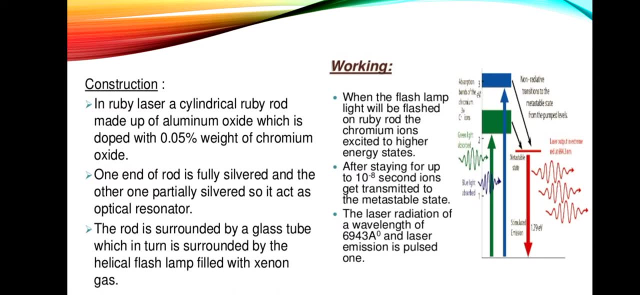 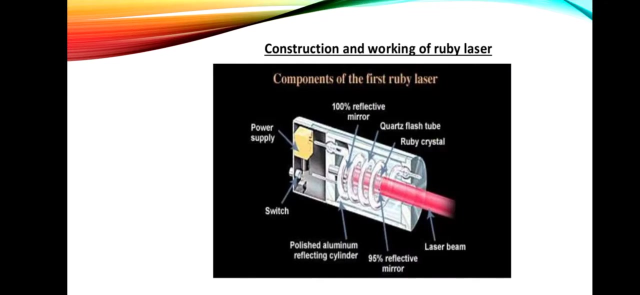 flash lamp filled with xenon gas. let us see the working of this, Louania Zer, when the splash lamp light will be flashed on Ruby Lord chromium ions excited to higher energy states after staying for up in higher energy state, after staying for update of minus eight seconds, I want to get. 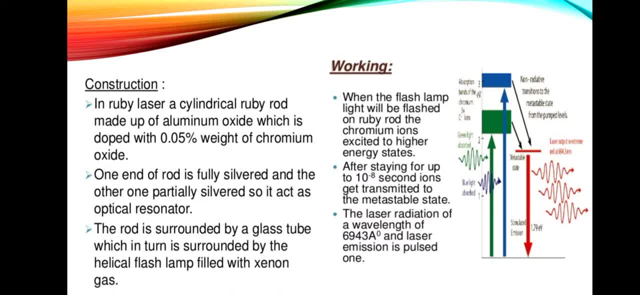 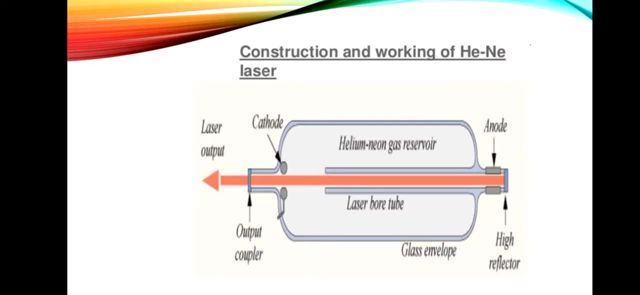 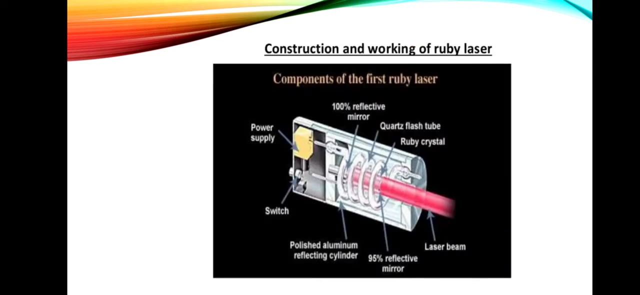 transport into metastable state. the laser radiation of a wavelength of 6,943 angstrom and laser emission is pulsed to 1. next next one here: gas laser. the example of gas laser is Zivoto and helium neon laser. you can see about helium neon laser. 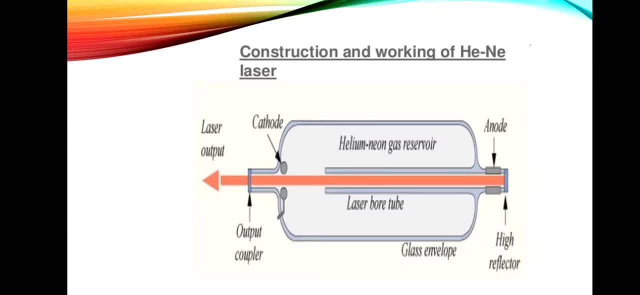 construction. this is the some manual of helium neon laser. this helium neon laser is a type of gas laser whose gain medium consists of a mixture of 10 is to 1 ratio of helium and neon at a total pressure of about 1 torr inside of a. 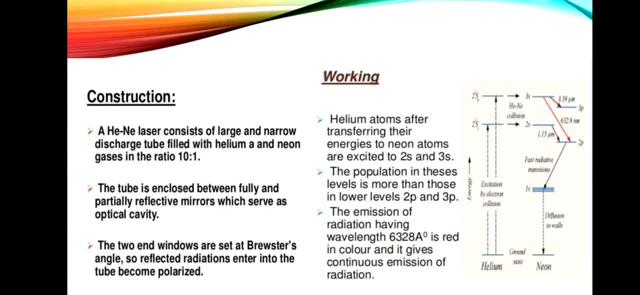 small electrical discharge. and this helium neon tube is enclosed between fully and partially reflective mirrors, which serves as optical cavity. this optical cavity, it describes an arrangement of mirror that produces a standing light wave resonator and the two end windows are here. there are two end windows right. this two end windows are set at Brewster's angle I. 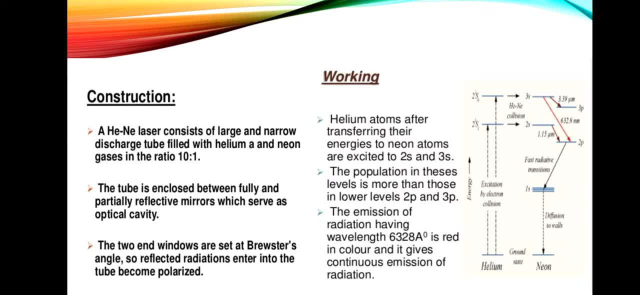 know you came the word across the board. Brewster's angle in your plus 2 means it is an angle of incidence at which light with a particular polarization is perfectly through a transparent dielectric surface with no reflection. okay, the angle of incidence that produces 90 degrees angle between reflected and refracted ray is called. 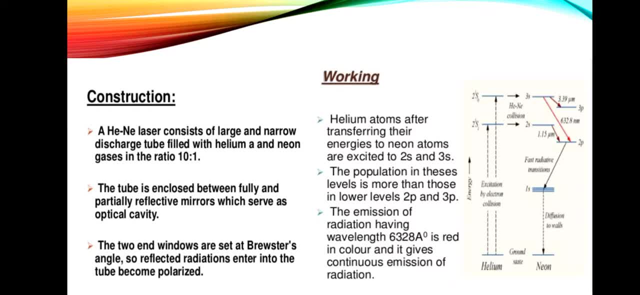 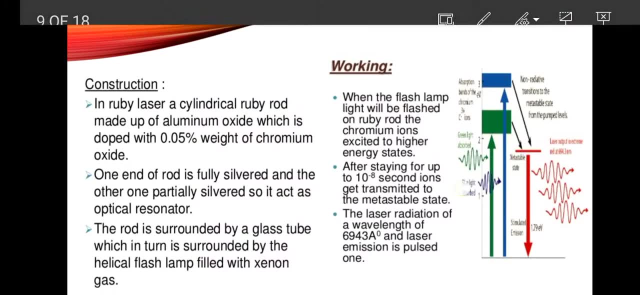 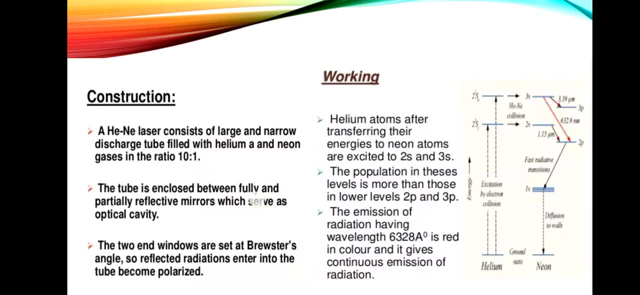 Brewster's angle. so the reflected radiations- so the reflected radiations enter into the tube- become polarized. next let us see the working of this helium neon laser. helium atoms, after transferring their energies to neon atoms, are excited to 2s and 3s after transferring the energies of. 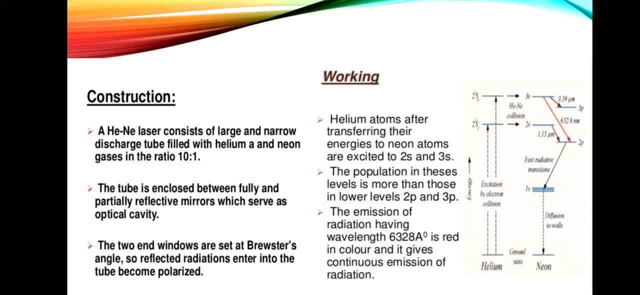 helium to neon. it was excited to 2s to 3s. okay, the population in in thesis levels is more than those in lower levels, 2p and 3p. this emission of radiation having 6,328 angstrom, as here, is in red in: 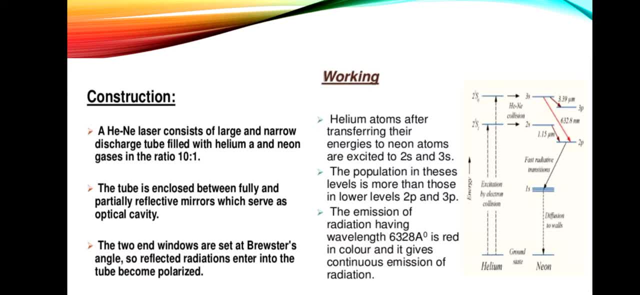 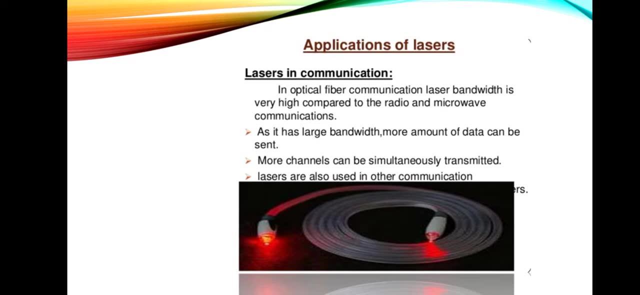 color and it gives continuous emission of radiation from 3s to 2p. okay, here are some. let us see some applications of lasers. lasers are all used in different fields. like first, lasers are used in communications. in optical fiber communication, laser bandwidth is very high compared to the radio and microwave communications, as lasers has a large 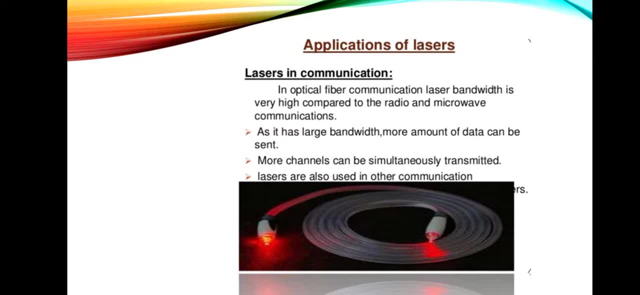 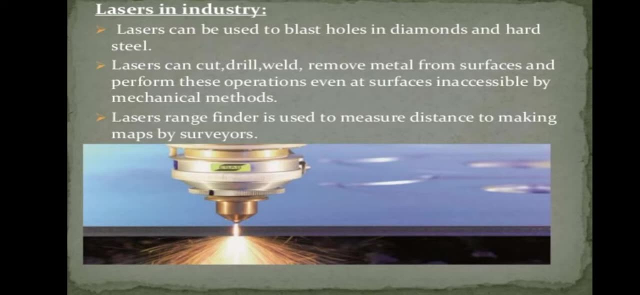 bandwidth, more amount of data can be sent. so lasers will used in this communication. well, are the advantages of laser in industry. laser in industry can be used to be a status in time. and then hard seems laser systems range I would in, primarily for pumping, plastic welding and sold in the 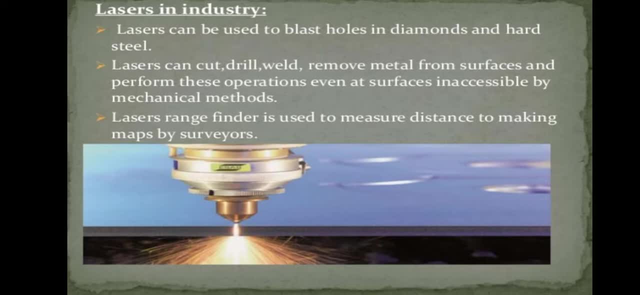 implications. higher power applications. the jasp have been cladding and deep and rating whirling. the quite might be killed for our kilowatts of optical power and are used in broad range of industrial processes. lasers rangefinder is used to measure distance to making maps by surveyors and 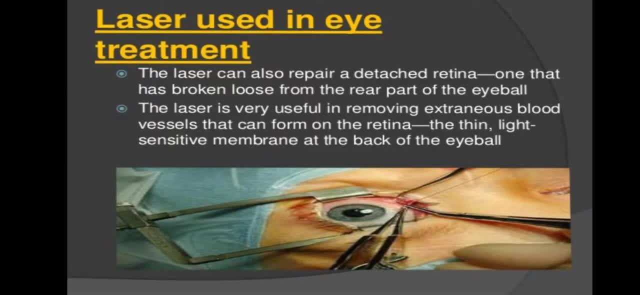 lasers used in medical treatment. medical treatment- lasers used in eye treatment- I mean laser eye surgery- is a medical procedure that involves the use of laser to reshape the surface of eye. this is done to improve or correct short sightedness or long sightedness. the laser is very useful in removing extraneous blood. 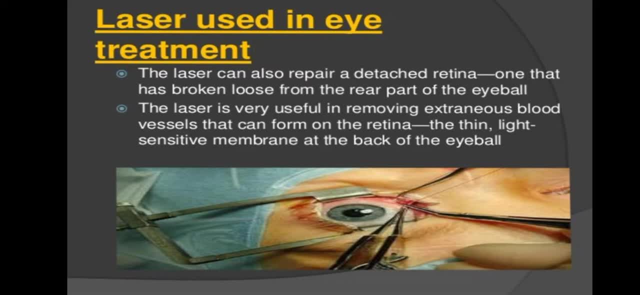 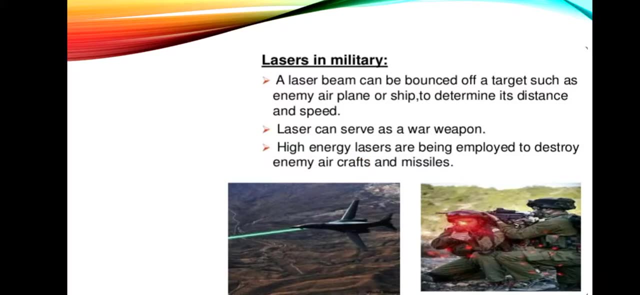 vessels that can form on the retina. lasers in military. military use of lasers is a laser target designator. this is a low power laser pointer used to indicate a target for a precision guided munition, typically launched from an aircraft. it can serve as a war weapon. the lasers are being 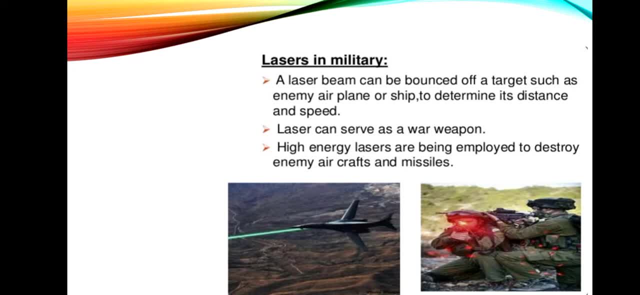 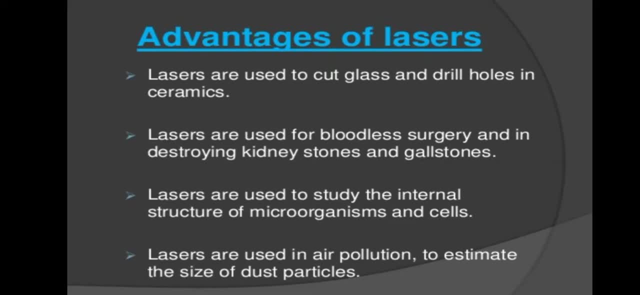 employed to destroy enemy aircraft and missiles. and here are some advantages of the laser. laser are used to cut glasses and drill holes in ceramics, and it is used as for hardening cladding pen and welding like that. and lasers are used for bloodless surgeries too, in destroying kidney stones and gallstones, and these.